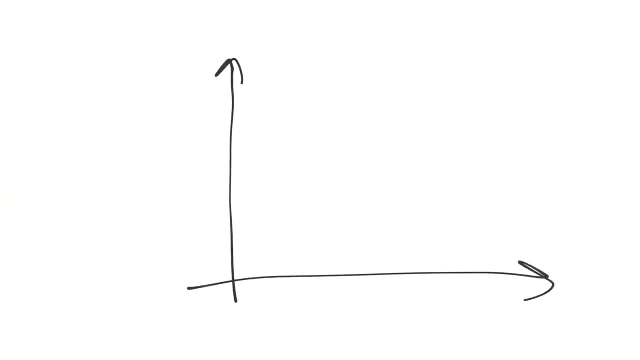 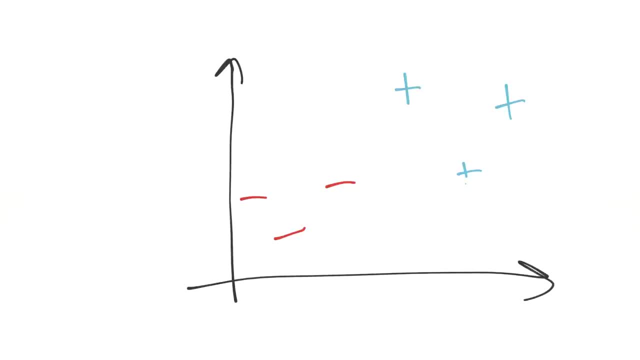 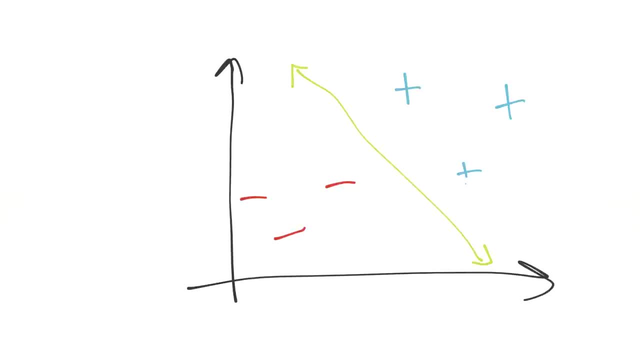 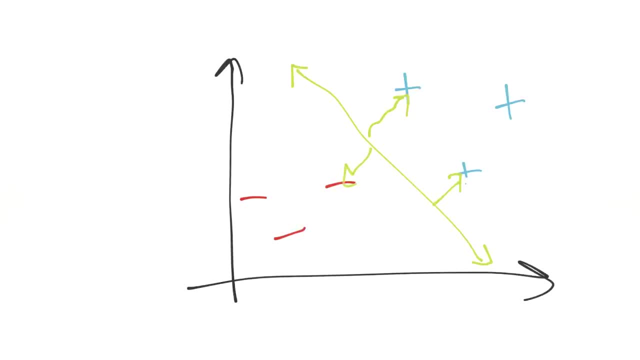 and this: okay, that distance is the greatest distance that you could come up with with a separating hyperplane. So, for example, another separating hyperplane might be this. right, That's a separating hyperplane. But the distance, again, the perpendicular distance between those is this: 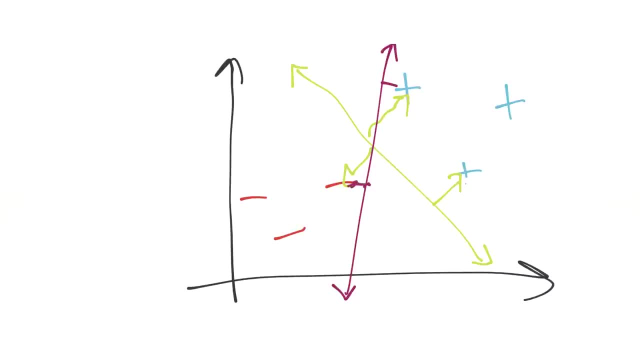 and like, oops, this right. Much smaller than our greenish-yellow counterparts. okay, So the support vector machine says that yellow-greenish line is the best separating hyperplane for our data. Now how we get to that is another story, but for now let's just remember. 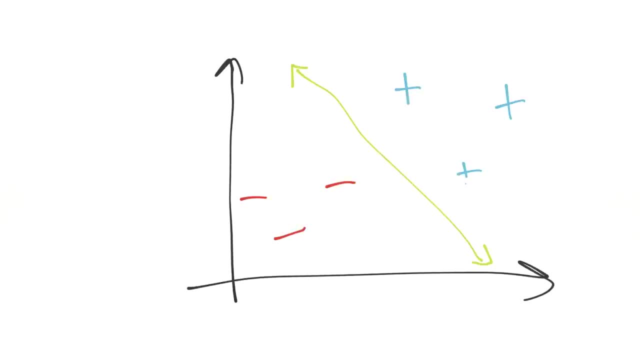 that is the- let's say that's the best separating hyperplane. Once you acquire the best separating hyperplane, you can now take in unknown data. So let's say you have an unknown data point, So unknown u, Because that u rests on the right-hand. 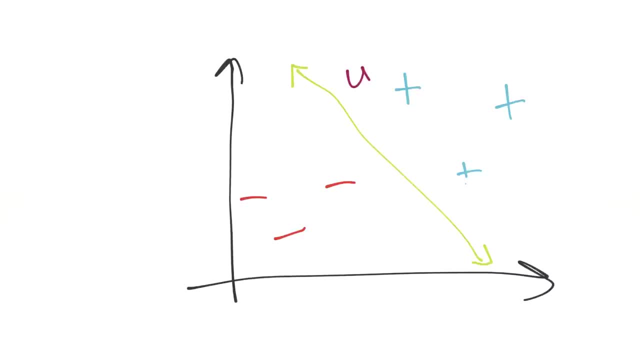 side of that separating hyperplane, we're going to say it's not unknown, It's a positive sample. Conversely, if you had an unknown that was down here, it's not unknown, It's on the left-hand side of this hyperplane. Therefore, it's actually a negative sample. So that is the intuition of 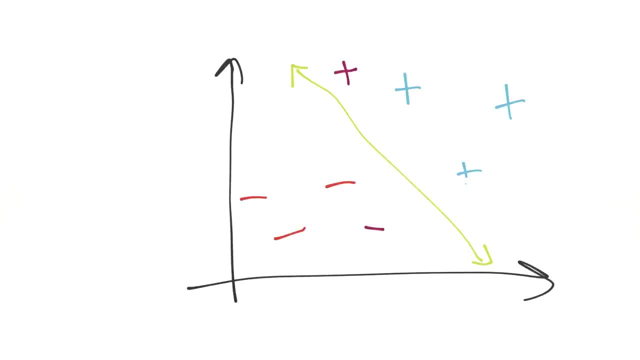 the support vector machine. We just need to find the best separating hyperplane and then from there we can classify new data points. Again, I will just reiterate: it's a binary classifier and natively it's a binary classifier. So if you have a binary classifier, you can classify new data points. 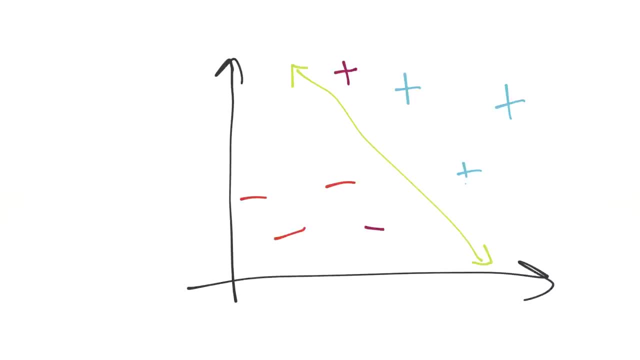 We want it to be against linear data. So, for example, what is the best separating hyperplane? Well, turns out we can't do that. Where is that hyperplane? It doesn't exist. So in theory you can't have one. but wouldn't it be nice if we could do like? 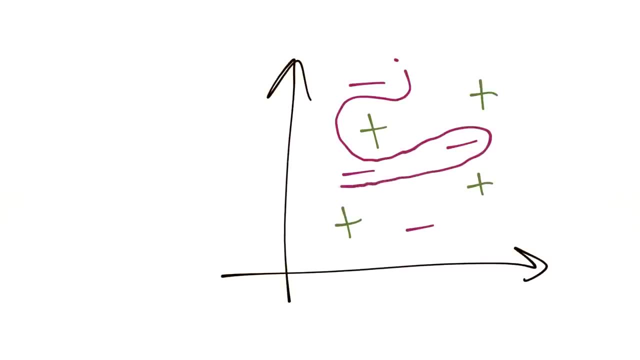 like that. Everything that is on the left side of this hyperplane is going to be against linear data. Everything that is on the right side is a plus, So I'll leave it to you to determine whether or not that's even possible, and we will answer that question, I promise, But for now, let's actually 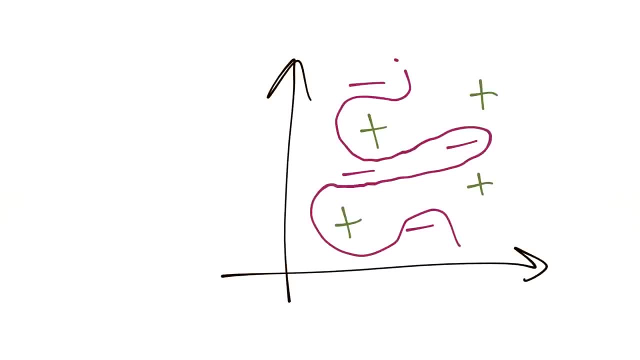 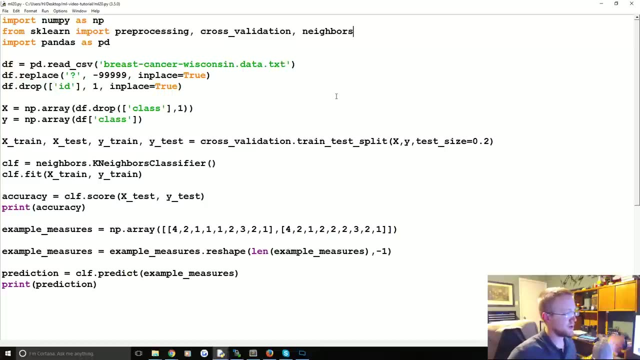 apply the support vector machine in a more simple example. We're going to be using the same example that we did before with the breast cancer data set, So let's go ahead and hop over there. Okay, so now what we're going to do is we're going to take the same code we used back in part 14. 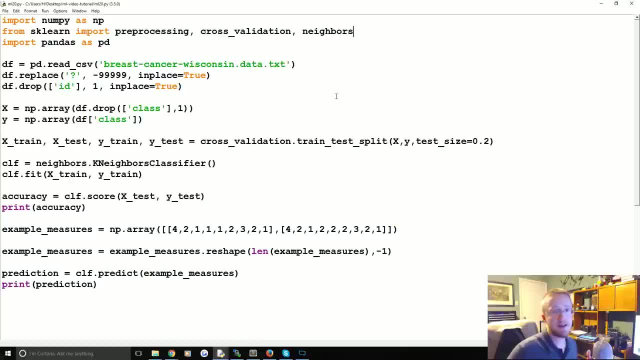 with the k-nearest neighbors algorithm. If you don't have that, go to the text version of this tutorial on pythonprogrammingnet and you can just copy and paste. It'll be right at the top. So here's the code. This is the code we used with the k-nearest neighbors. Now, using the support: 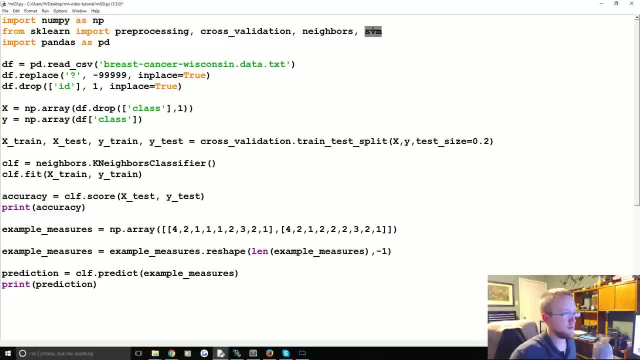 vector machine. super simple. We're going to import support vector machine from sklearn and then we're going to come down to the classifier, and we're not going to be using k-nearest neighbors, We're going to use svmsvc for support vector classifier. 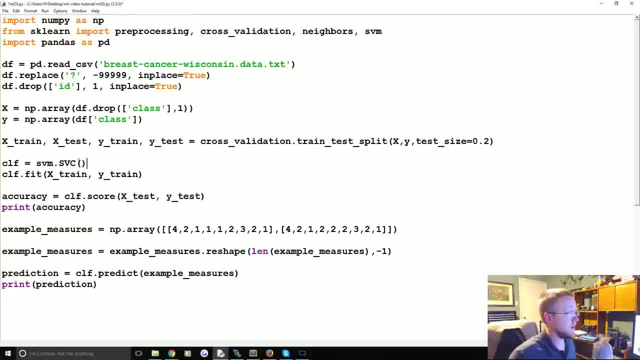 and then we're going to use empty parameters. there There are a lot of parameters that we can modify, but in order to know what to modify or what it's doing, we need to break down the algorithm first. So for now, we'll just use the defaults and let's go ahead and run it. 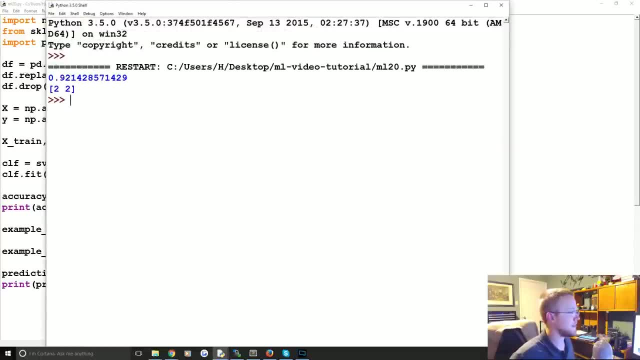 because that's all we have to do, Super simple, to change algorithms. So there we go. We ran it- 92% accuracy. and then this is the classification that we just kind of made up and it did it right. Let's run it one more time. 92 seems kind of low. There we go, 96. Okay. 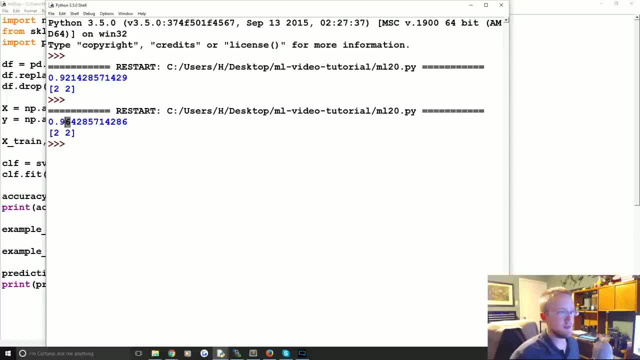 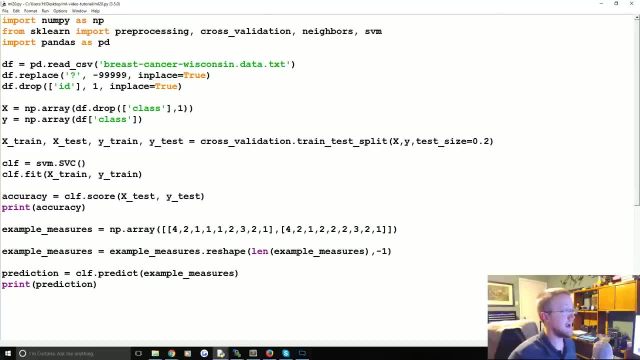 so that is the support vector machine in practice. Again, all we did was just take the data, replace some of the data with some outliers, which later now you'll see how different the support vector machine handles outliers as opposed to the k-nearest neighbors. What if we did not? 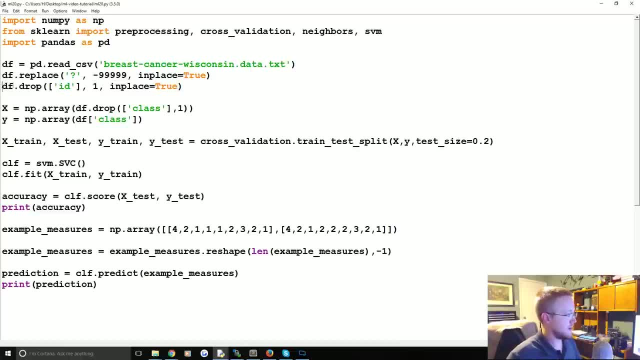 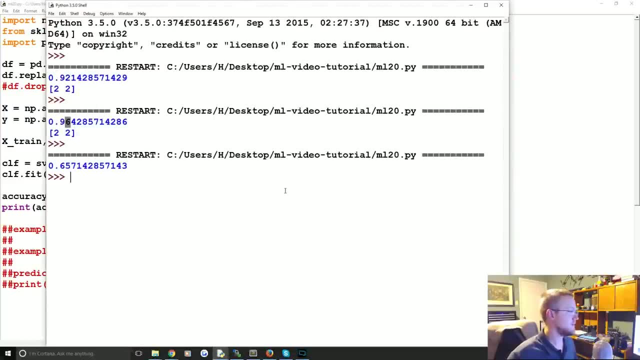 drop the ID column, So let's do that, and then we're just not going to make a prediction. So if we don't drop the ID column, we're relegated back to about 60%- 95% accuracy. So it does better than the k-nearest neighbors did when we left in the ID column. 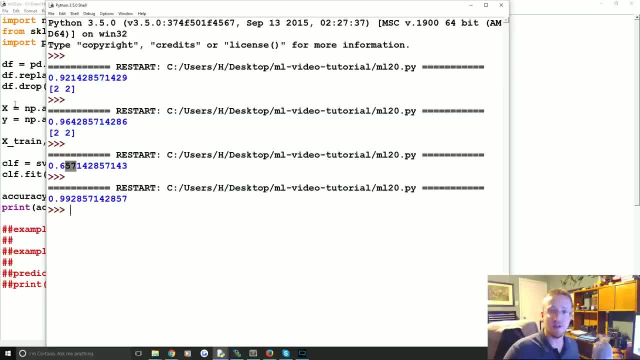 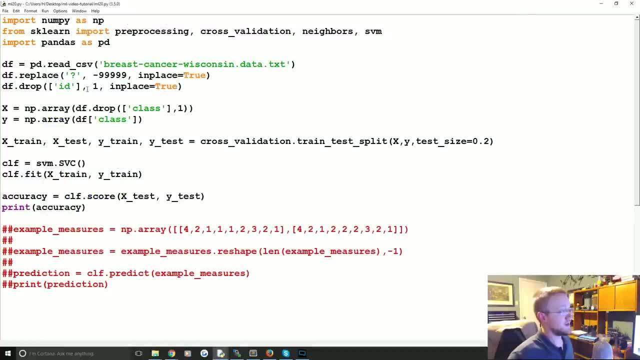 but it still has a huge impact. So ID was just kind of a useless data column. Oh, that time we got 99% accuracy, Nice, Anyway. so that's that, Anyway. so we dropped the ID column, so it's. 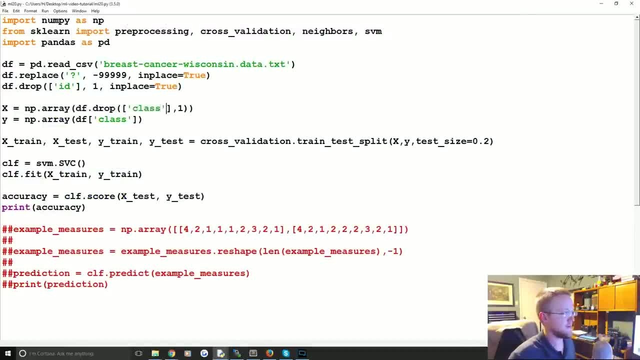 useless. and then our Xs are just everything except for the class. So our features are everything but the actual label itself. The Ys are our label. We do the train test, call the classifier, train the classifier and then test it. Okay, simple enough. So 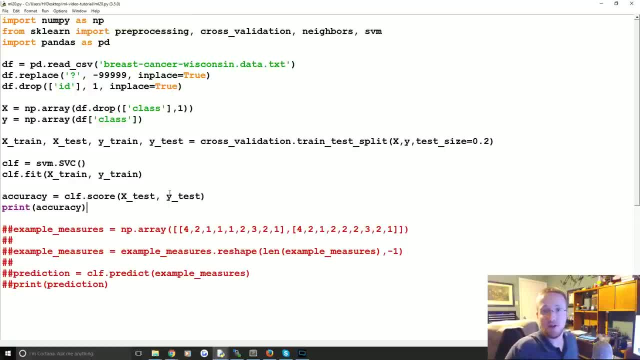 that is the theory and application of a support vector machine. Now we're going to break it down, So if you have any questions, comments, concerns up to this point, feel free to leave them below. Otherwise, stay tuned to the next video. Thanks for watching.